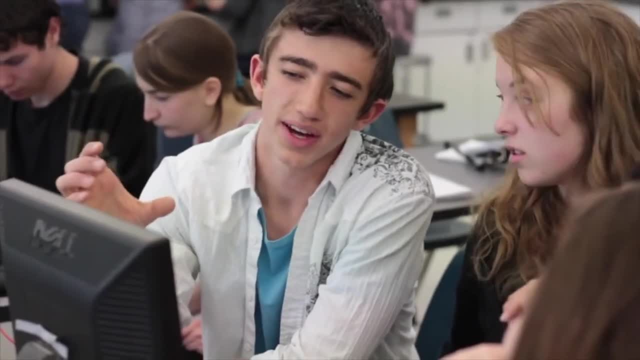 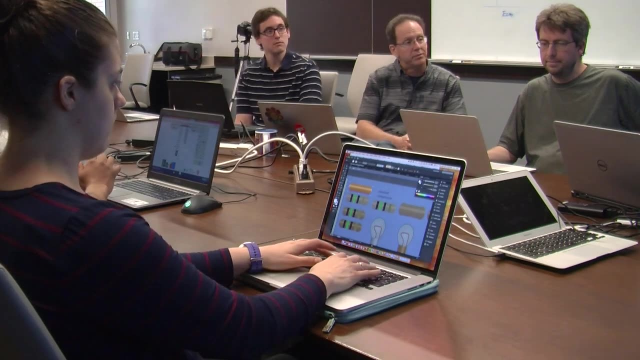 predictions and conjectures and to really take ownership over their learning. PhET's work over the past 17 years in science provided us with a rich research base around simulation design and evidence of how simulations can impact science learning. In this grant, we 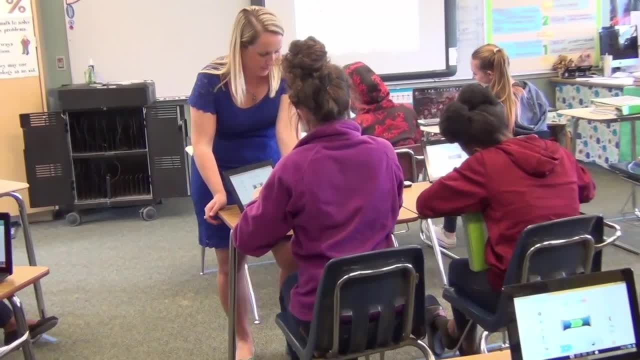 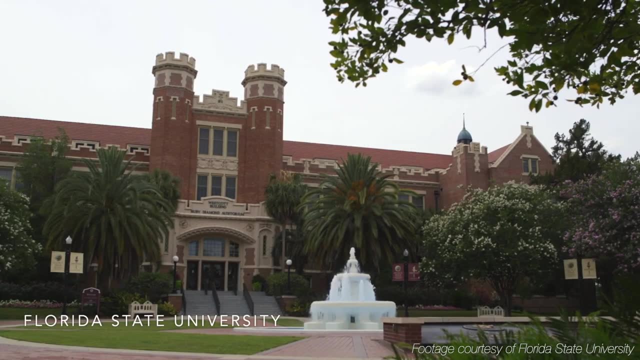 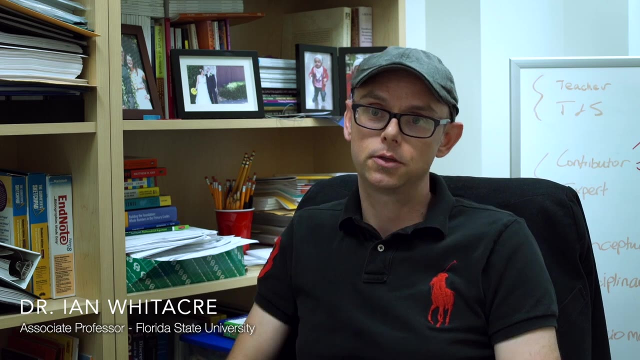 teamed up with mathematics education researchers to look specifically at simulation design around mathematics and how these simulations can impact classroom teaching. In a traditional math classroom the dynamic tends to be: a lot of information is coming from the teacher or the textbook and students are essentially expected to memorize and repeat that back With PhET interactive. 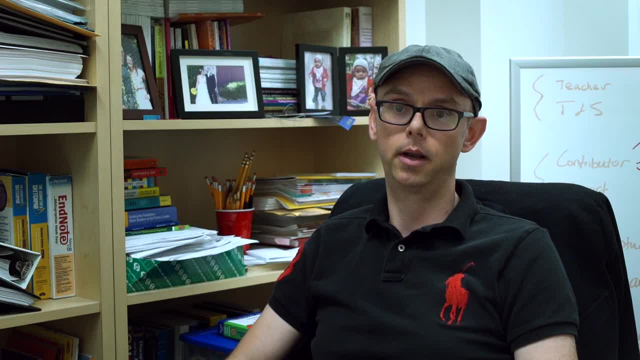 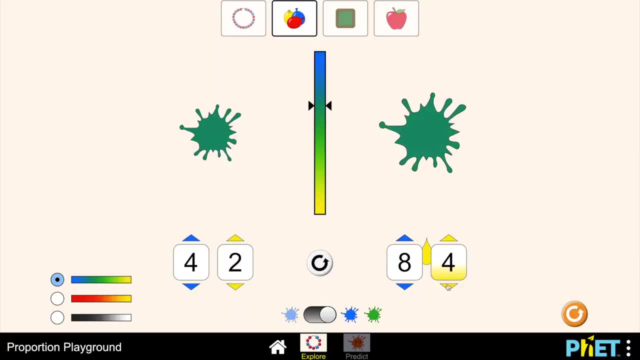 sims, there's a lot more potential for students to develop the mathematics on their own because they have the chance to explore and experiment with an environment in which they're getting feedback and they can come to an understanding of what the mathematical or the scientific 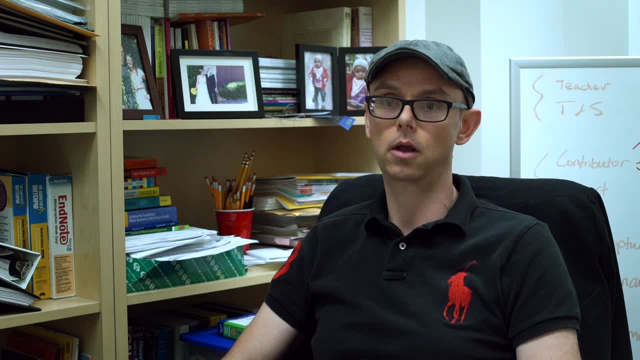 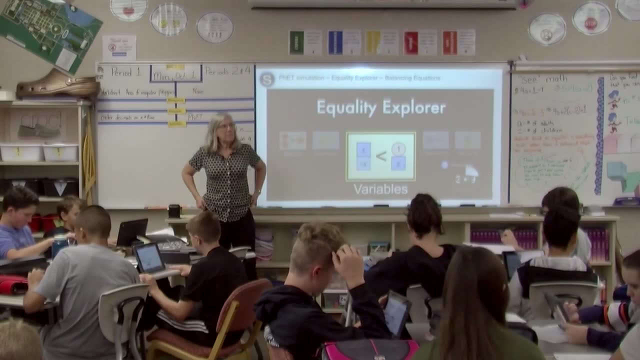 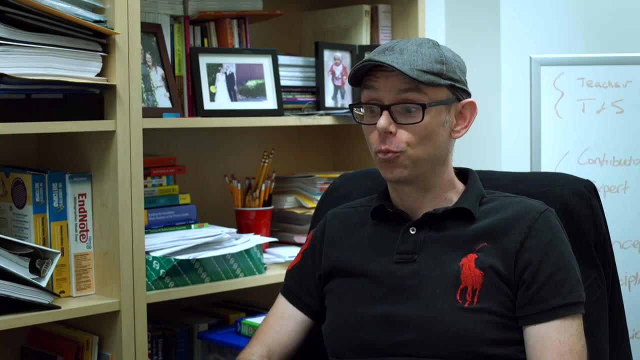 relationships are. So in this study we were really interested in the contrast between the PhET sim lessons and the regular math lessons within the same teacher's classroom. You are to come up with, minimally, to teach me five things about this tool that I don't already know. We found significantly different. 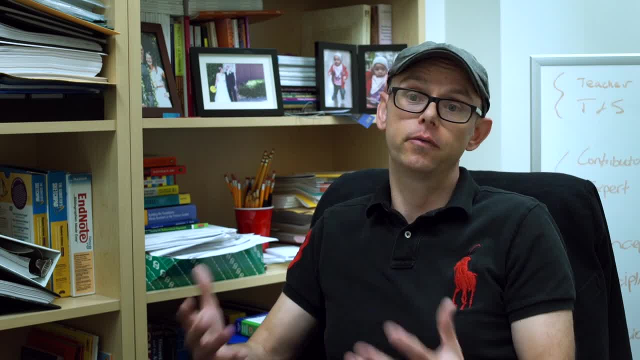 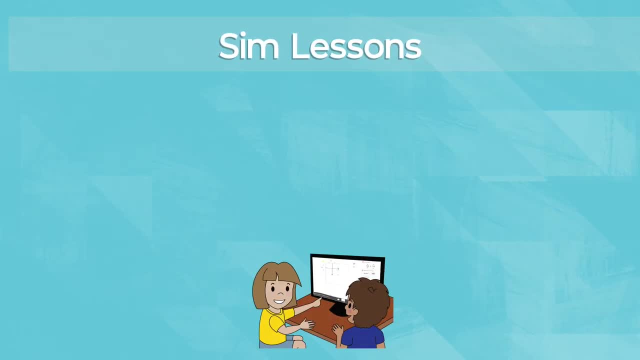 norms in those two types of lessons, meaning the nature of the activity was different and the expectations for students engagement in mathematics were different. Specifically, in the sim lessons, students were exploring new mathematical ideas, they were inventing strategies and they were sharing their 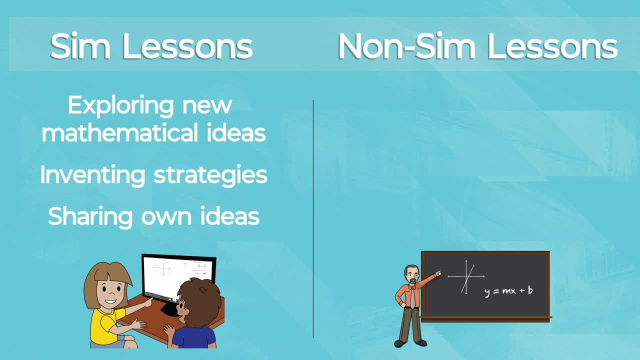 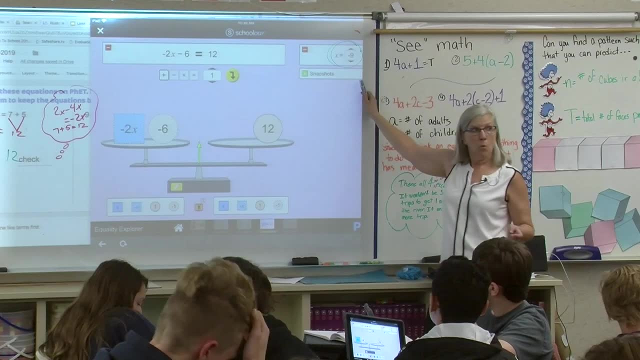 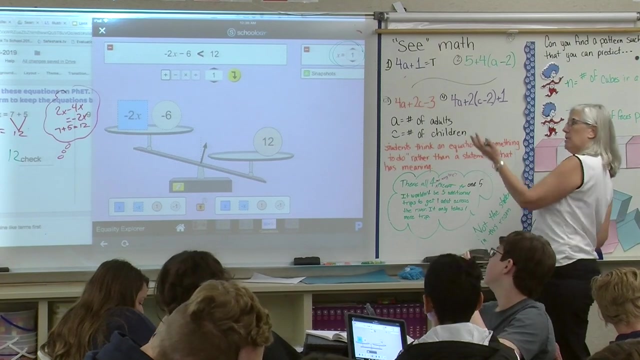 own ideas, Whereas in the non-sim lessons they tended to be much more focused on practicing standard procedures, recalling facts and generally preparing for tests. Well, you take that back up high again. How did what happened when that was shifting to the regular math? 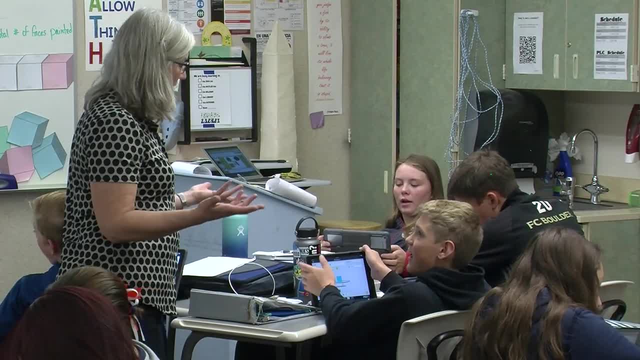 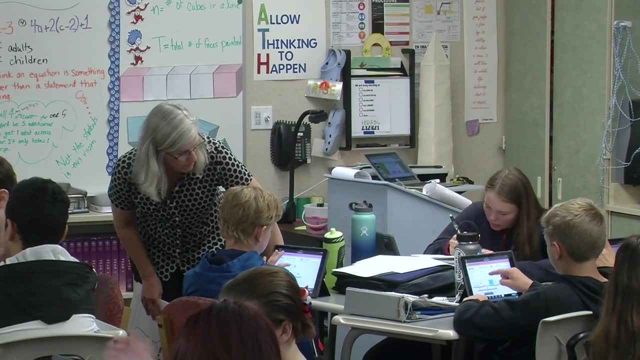 Well, the findings of this study illustrate that PhET sims can can play a powerful supportive role in engaging students in mathematical practices and shows that there are teachers who may be teaching in pretty authoritative, teacher-centered ways typically, but with the use of a material like a PhET sim. 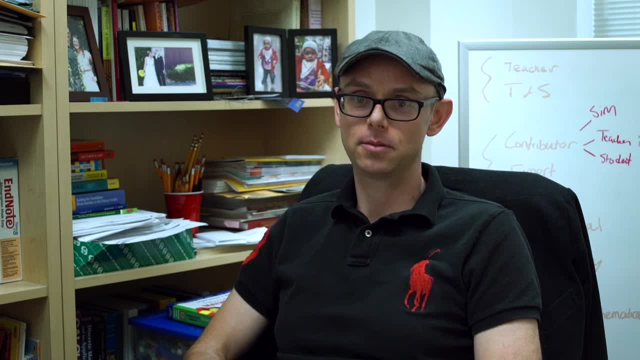 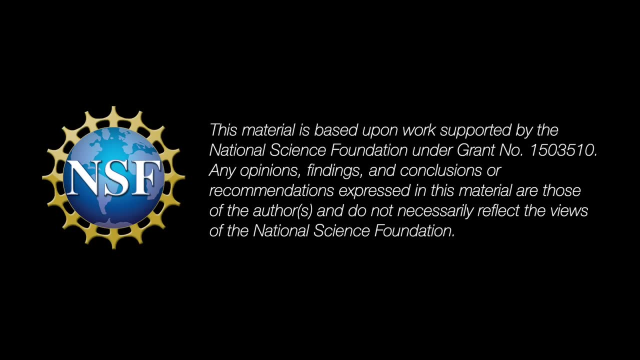 their classroom can be transformed and they can engage students in mathematics in these powerful ways. you